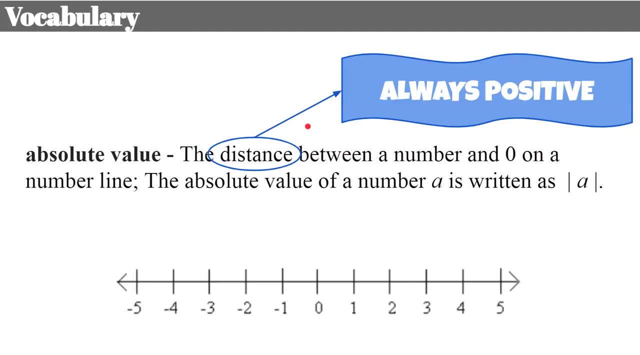 from somewhere. you always use a positive number. When you get there, you don't say that you're negative miles away from where you were. You're still so many miles away, So it's a positive value. Now let's look at the absolute value of negative five. 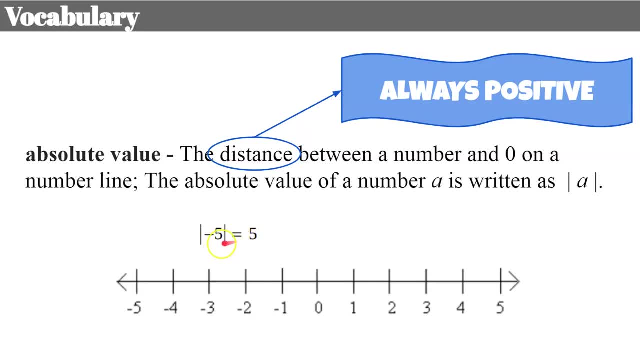 That is equal to positive five. And let me prove to you why. If I graph negative five on this number line, the distance that it is from zero is five. So it's five units away. So the absolute value of negative five is five. If I graph positive five, it is also five units away from zero. It doesn't. 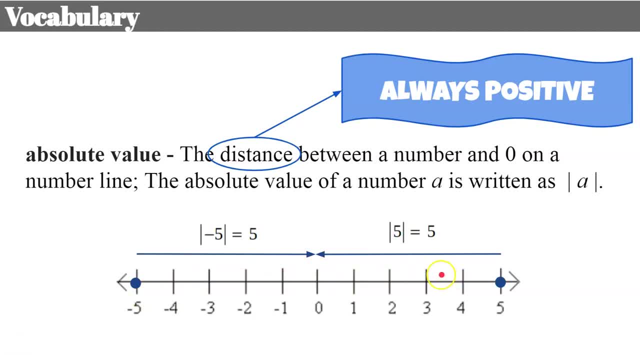 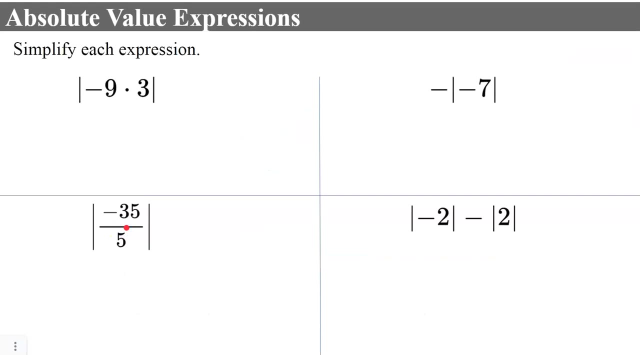 matter that I'm on the left or the right, The distance that it is from zero is five. So that is how absolute value is proven, And remember, the absolute value of anything is always a positive amount. So now let's review absolute value and make sure you understand that. 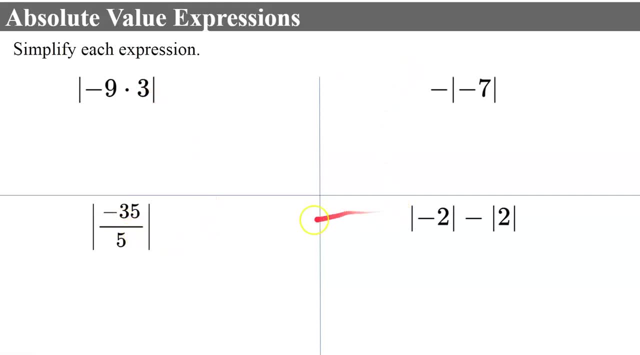 So I'm going to ask you to pause the video here and simplify these four expressions. Please come back and hit play when you're ready. Welcome back. So I hope you evaluated inside the parentheses first. So the first thing I'm going to do is multiply Negative. nine multiplied by three is negative. 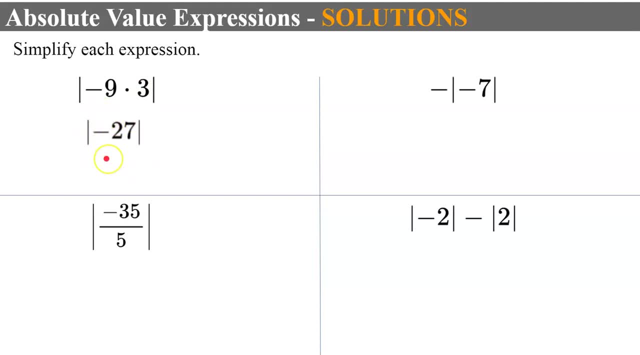 twenty-seven. Now I'm going to find the absolute value of negative twenty-seven, which is positive twenty-seven. Here we have negative absolute value of negative seven. You can also imagine there's an invisible one here. So negative one multiplied by the absolute value of negative. 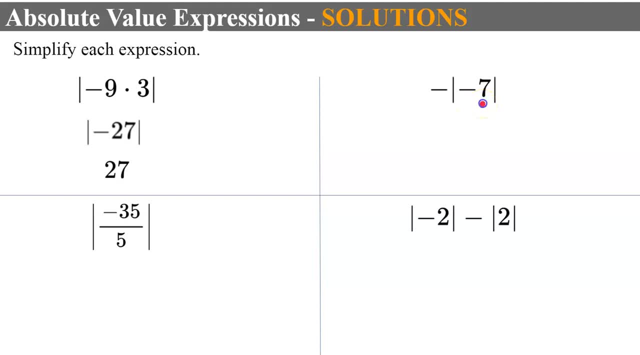 seven. So the absolute value of negative seven is seven And negative one times. the absolute value of seven is negative seven, Or think of it as negative seven, because the absolute value of this is seven. Over here we have negative thirty-five divided by five, which is negative seven, And then the absolute value of 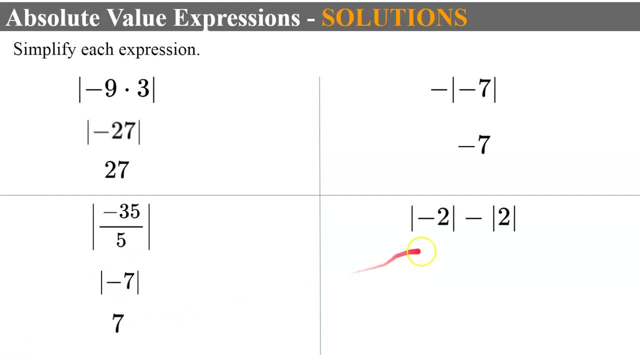 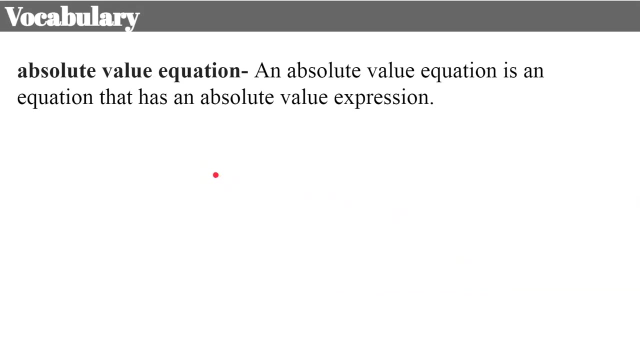 negative seven is positive seven And, last but not least, the absolute value of negative two is two and the absolute value of two is two. Two subtract two is zero. Moving on to absolute value equations: An absolute value equation is an equation that has an absolute value. 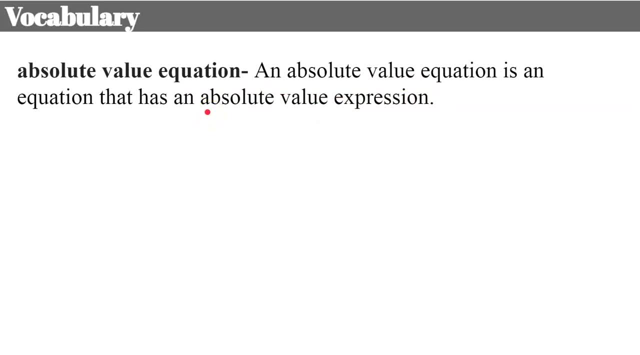 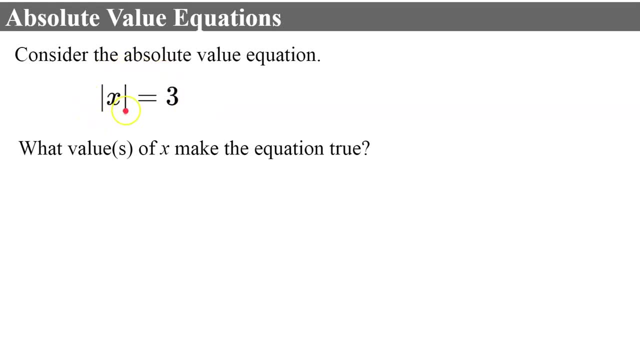 expression. So in the previous slide I showed you absolute value expressions. So here's an example of an absolute value equation. The absolute value of x is equal to three And we want to determine what value or values of x make this equation true. 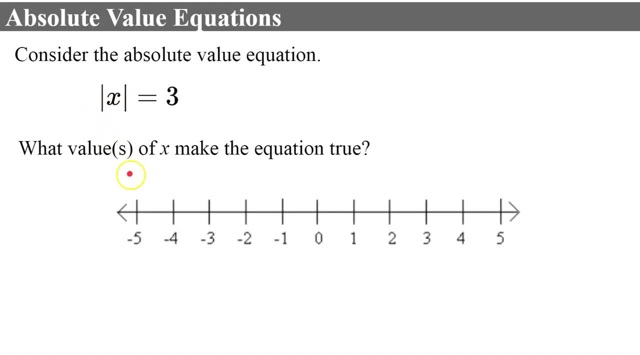 So I'm going to model this using a number line And we know that we're talking about a distance of three, So we're talking about absolute value. is the distance something is from zero. So imagine that what this is telling you is: x is three units from zero. 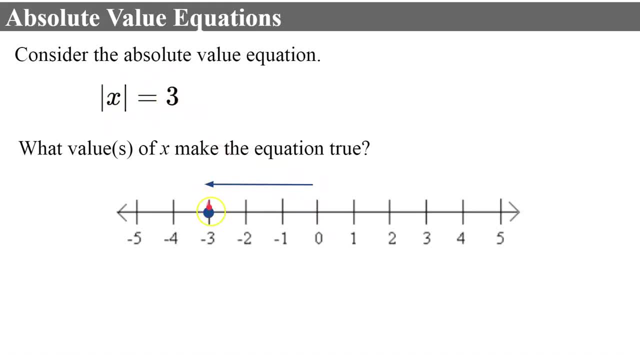 So if we look at it on a number line, we're going to go three units from zero. we get to negative three. But we can also go three units from zero to the right and get positive three. So therefore we can say that x is equal to- here's a symbol- positive and negative three. Some people write x equals negative three and three. or you could write x equals negative three and x equals three. 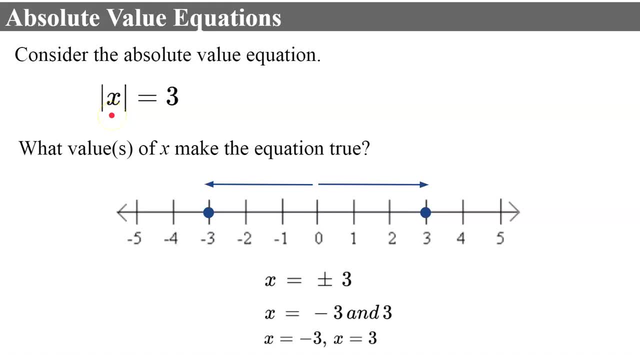 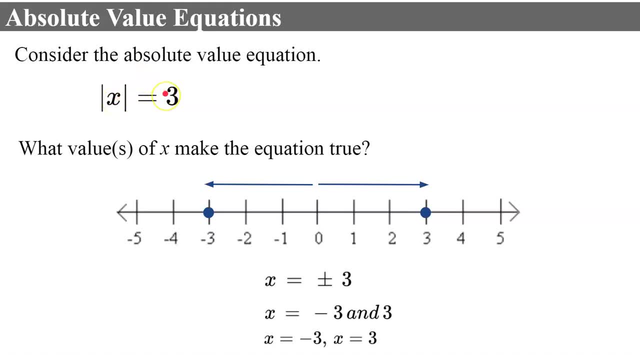 If I plug in three for x, the absolute value of negative three is positive three. If I plug in three for x, the absolute value of negative three is positive three For x, the absolute value of three is also three. So there are two different values that x could be and it still will be equal to three. 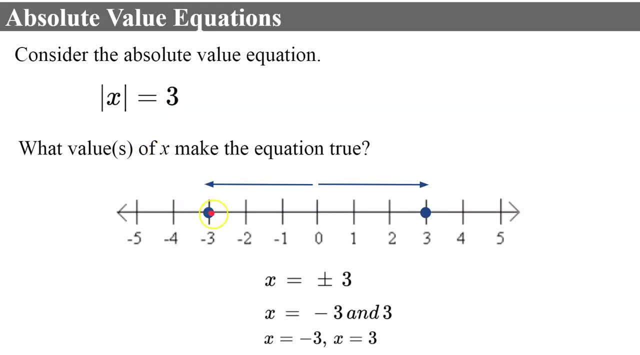 If you're ever asked to graph an absolute value equation, what you would do is just plot the two points on the number line, So you wouldn't connect or shade anything in between. There'd be no arrows, there'd just simply be one point and a second point. 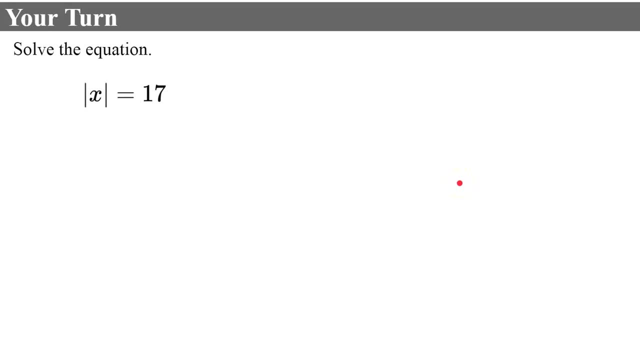 Your turn. I would like you to solve the absolute value equation. please pause and come back when you're done, welcome back. so our solution for this would be negative 17 and X equals 17. so it's and it's two different values. the absolute value of negative 17 is positive 17 and the absolute value of 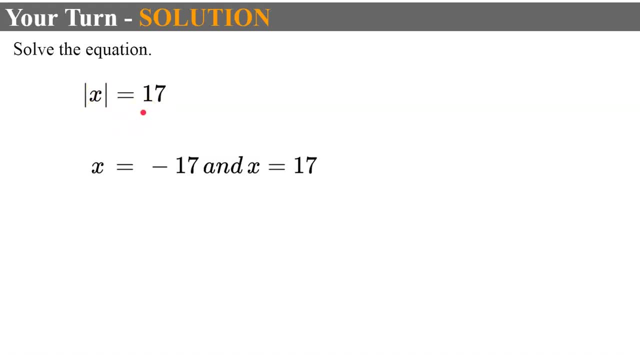 17 is also positive 17. so our solution is: X equals negative 17 and X equals 17. now we're going to talk about solving an absolute value equation that has an expression inside the absolute value. so for a minute I want you to think about. 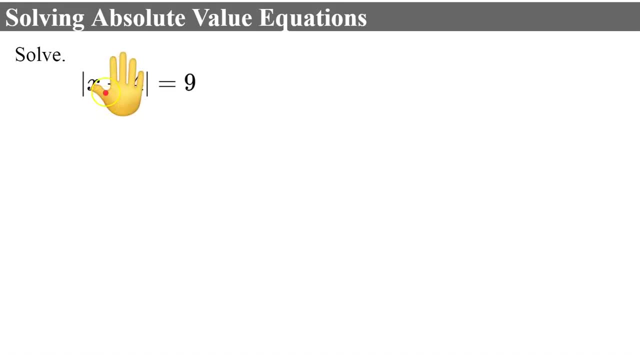 this. let's cover up what's inside. it doesn't really matter. as we start to set up, we know that whatever is inside this absolute value expression can be equal to negative 9 and it can be equal to 9. so whatever is inside the absolute value expression- remember it can be equal to negative 9. 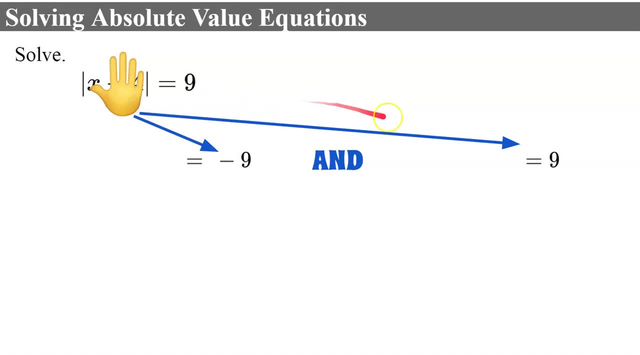 because the absolute value of negative 9 is 9 and the absolute value of 9 is 9. so now we'll uncover it and now we know that X plus 4- is what is in the absolute value- can be equal to negative 9, seeing as the absolute value of this is. 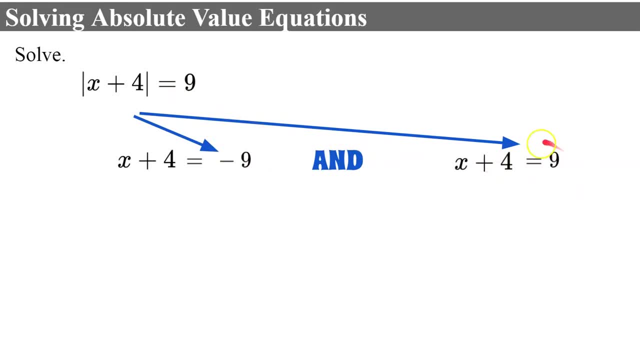 positive 9 and the X plus 4 could be equal to positive 9. so now we're going to solve each of our equations. we're going to subtract 4 from each side, because the inverse of add 4 is to subtract 4, giving us a solution of X equals negative 13, negative 9 and 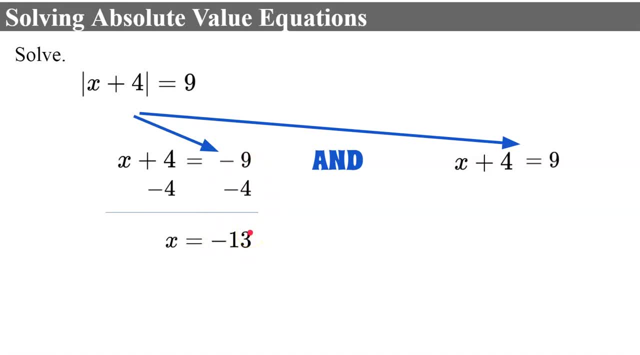 negative 4 are negative 13. let's check this. negative 13 and for X: negative 13 plus 4 is negative 9. the absolute value of negative 9 is positive 9, so it checks. now let's solve our second equation. we are going to subtract 4 from. 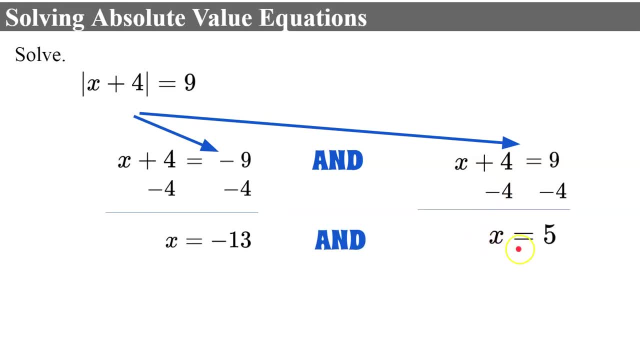 each side, giving us a solution of X is equal to 5, since 9 subtract 4 is 5. let's check. we're going to come back over to our original absolute value equation. if X were 5, 5 plus 4 is 9. the absolute value of 9 is 9. so it checks, so our 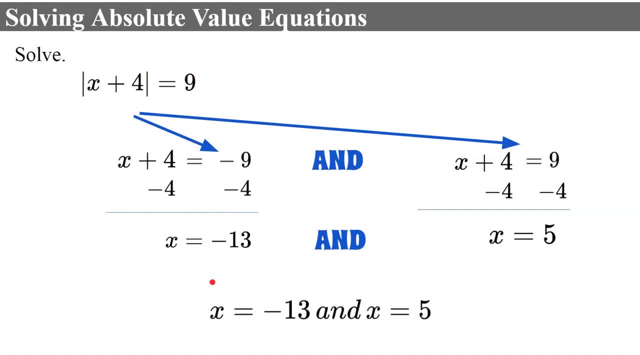 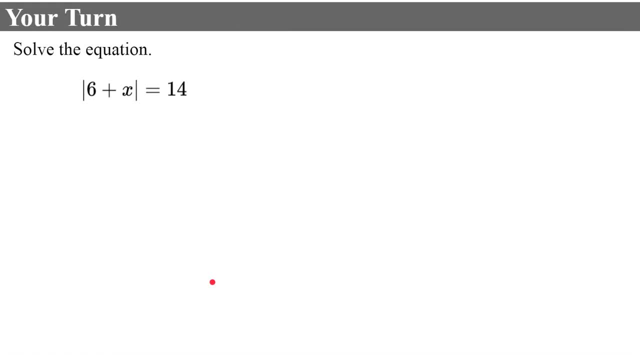 equations are: X equals negative 13 and X equals 5. your turn, go ahead, pause, write two equations, check your solution and come back when you're ready, welcome back. so here's our solution. so, once again, I doesn't matter what's inside my absolute value expression, but I know that it can be equal to negative 14 and 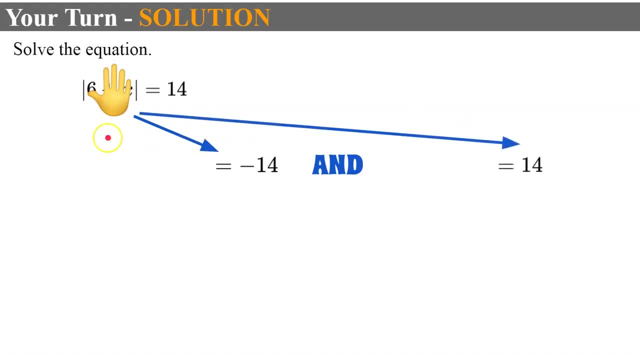 positive 14. now I can uncover what was in there and know that it's going to be 6 plus X. that can equal negative 14 and 6 plus X can equal positive 14. I'm going to subtract 6 from both sides. X is equal to negative 20. negative 14. subtract 6 is negative 20. 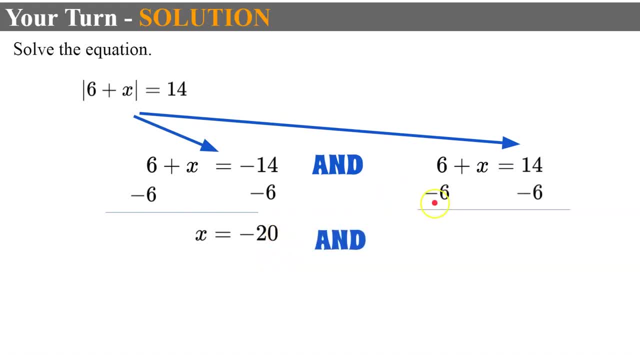 come back over here to my second equation: negative 6 subtract from both sides, and X is equal to 8. 14 subtracted 6 is 8.. Let's check If x was negative 20,, 6 plus negative 20 is negative 14, and the absolute value. 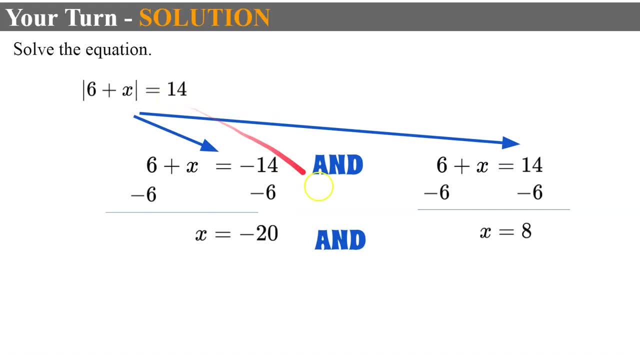 of negative 14 is positive 14.. Now we want to take our second solution of x equals 8.. Over here, if x were 8,, 6 plus 8 is 14, and the absolute value of 14 is positive 14.. So our solutions: 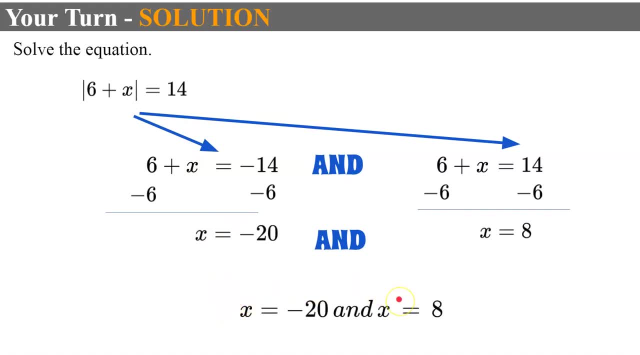 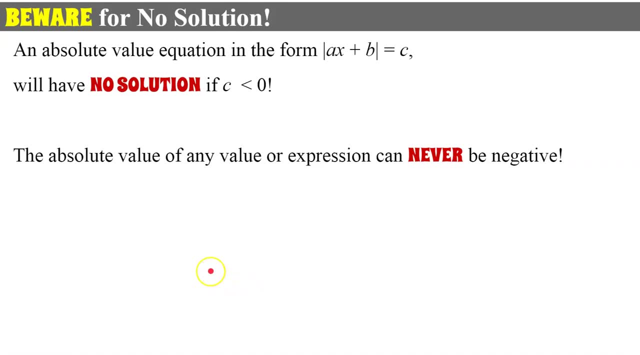 are x is equal to negative 20 and x is equal to 8.. One thing to beware of as you're solving an absolute value equation: An absolute value equation in the form the absolute value of an expression equals c will have no solution If c is less than 0. So if it's less than 0, that means c, that this equation is equal to a. 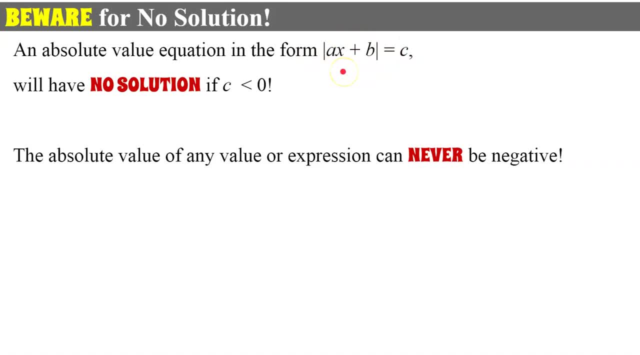 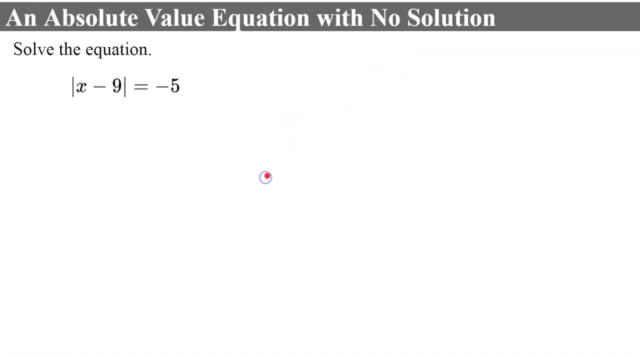 negative amount. The absolute value of anything will never be equal to negative amount, So it can never be negative. So here's an example We have: the absolute value of x subtract 9 is equal to negative 5.. So I can look at this. 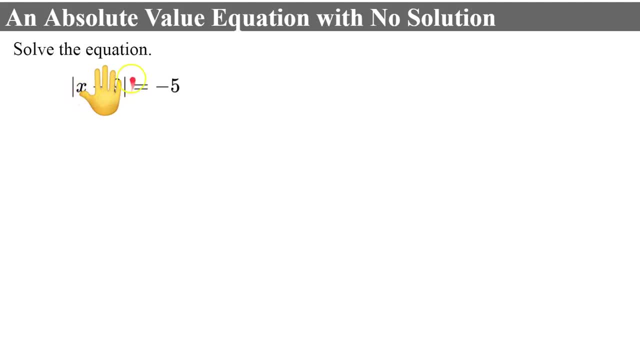 It doesn't matter what's inside the absolute value, because there is no value I could put inside this absolute value expression that would ever be negative, because absolute value represents the distance from 0, and distance is never 0, is never negative, so there's no value to make this ever equal to negative. 5. so therefore, because the 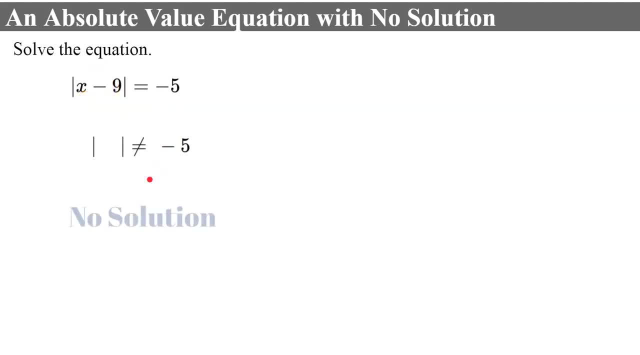 absolute value of nothing can't be ever be negative 5. we have no solution. there is no value for X. that will result: the absolute value of X minus 9 equals negative 5. no solution would be your answer. so be careful, because if you're not paying attention, you could still split this into two equations. get a. 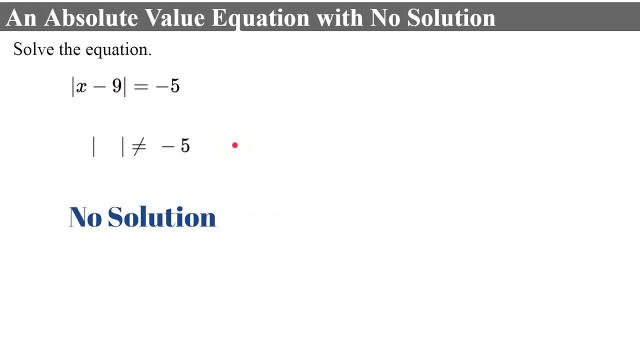 solution, but the solutions would not check. so it's really important for you to check your solutions and think before you split them into two equations. all right, let's do some practice before we close up this video. I'm going to go ahead and get started and I'll see you in the next video. 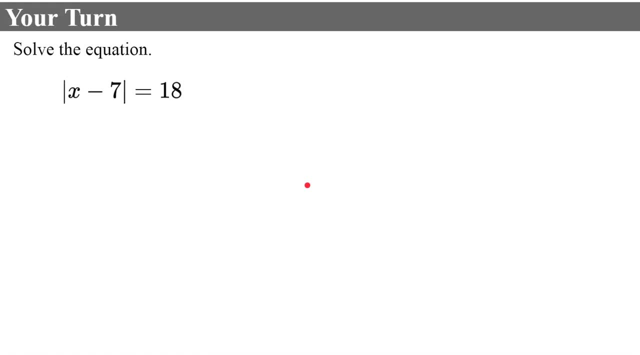 I would like you to solve this equation and come back and hit play when you're done. please pause, welcome back. so I hope you wrote the equation. X subtract 7 is equal to positive 18 and X subtract 7 is equal to negative 18. it doesn't matter. 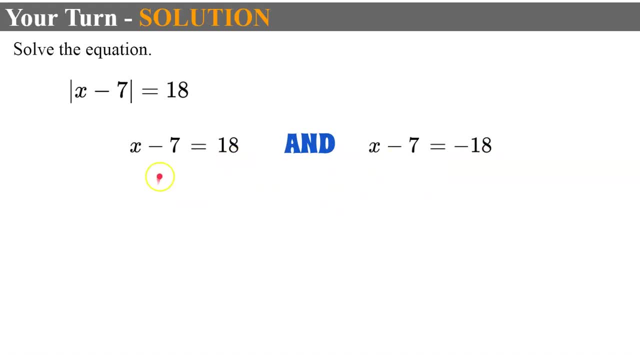 what order you wrote them in. you could have flip-flopped them. we're going to add 7 to both sides to solve, and X is equal to 25. let's check it: twenty five subtract 7 is 18. the absolute value of 18 is equal to 18. the 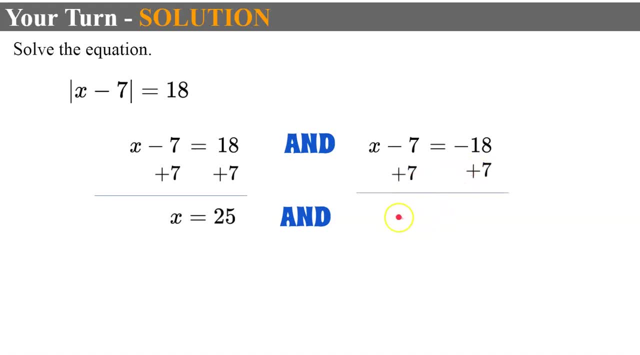 second one. we're going to add 7 to both sides and X will be equal to negative 11. negative 18 plus seven is negative 11. let's check it: if X is negative 11, negative 11, subtract 7 is negative 18. remember, add the opposite, negative 11 and. 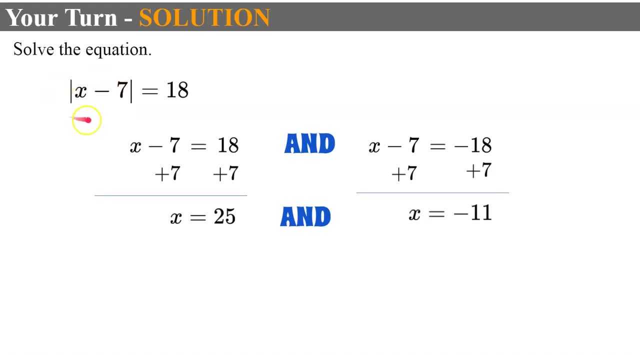 negative 7 is negative 18. the absolute value of negative 18 is positive 18. it checks. so our solutions are: x equals 25 and x equals negative 11. remember the order that you answer does not matter, meaning if you had x equals negative 11. 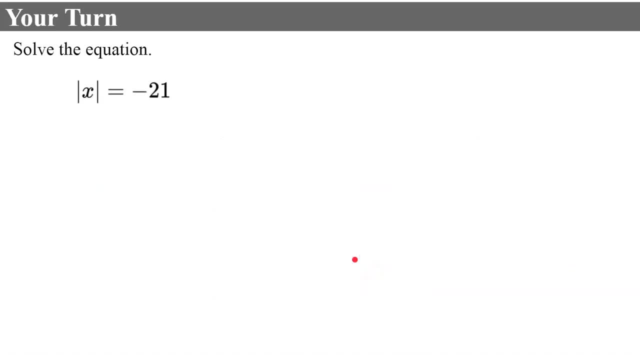 and x equals 25. try this one. please pause, come back when you're ready. welcome back. let's see how you did so. I hope you have no solution. the absolute value of X. there is no value for X that will ever result. the absolute value equals negative 21. your turn. please pause and come back when you're ready. 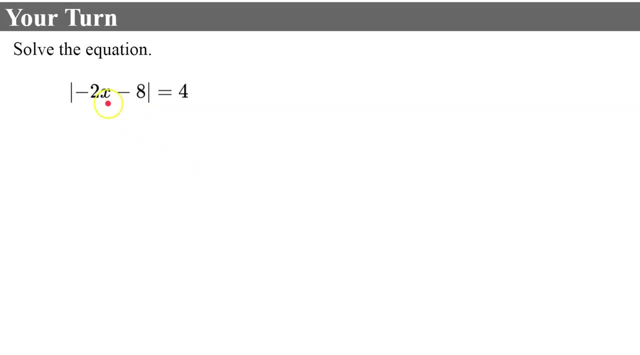 welcome back. let's see how you did so. we're going to split into two equations. the expression inside the absolute value signs can be written as negative 21, and negative 21 can be written as positive 21 equal to positive 4, and the expression inside the absolute value can also be. 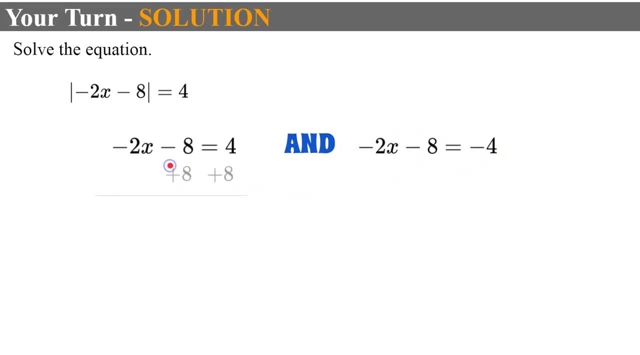 equal to negative 4. we're going to solve by adding 8 to each side, giving me negative 2x equals 12. divide both sides by negative 2 to solve for X and X is equal to negative 6. let's check this. if X were negative 6, that'd be negative 2. 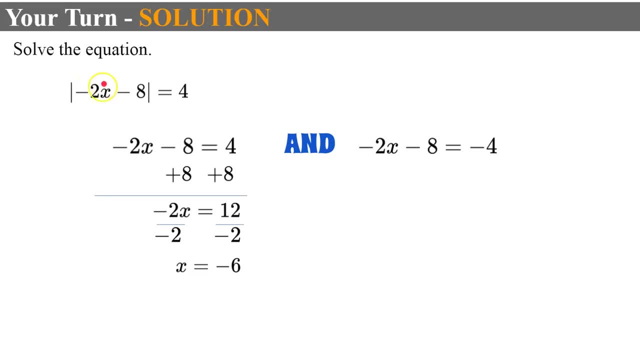 times negative, 6, which is positive, 12, positive, 12 subtract 8 is 4. the absolute value of 4 is 4. and our second equation: let's add 8 to both sides, giving us negative 2x is equal to 4. negative 4 plus 8 is. 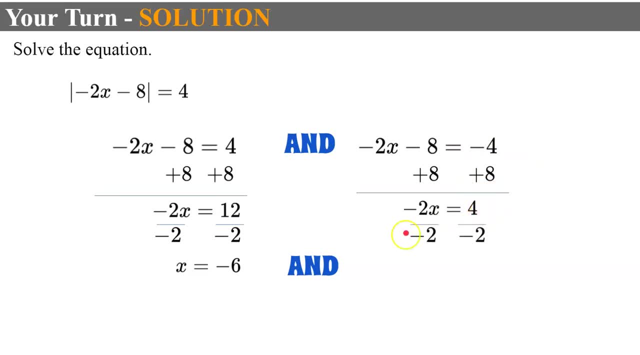 positive 4, divide both sides by negative 2 and X is equal to negative 2. 4 divided by negative 2 is negative 2. now let's bring this back up. check If x is negative 2, negative 2 multiplied by negative 2 is positive 4.. 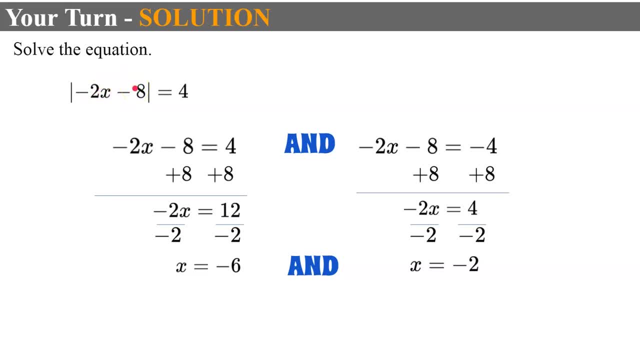 4 subtract 8 is 4, add negative 8 or negative 4.. The absolute value of negative 4 is positive 4 and it checks. So our solutions are: x is equal to negative 6 and x is equal to negative 2.. So there you have it. That's solving. 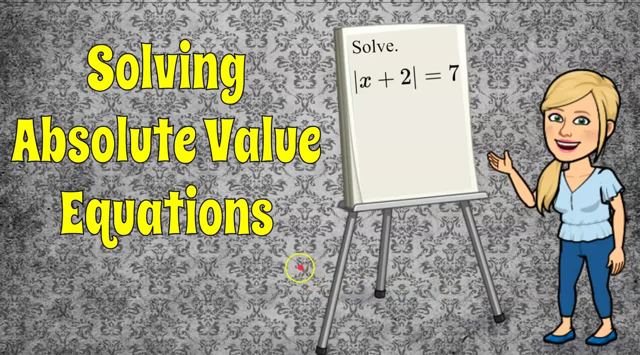 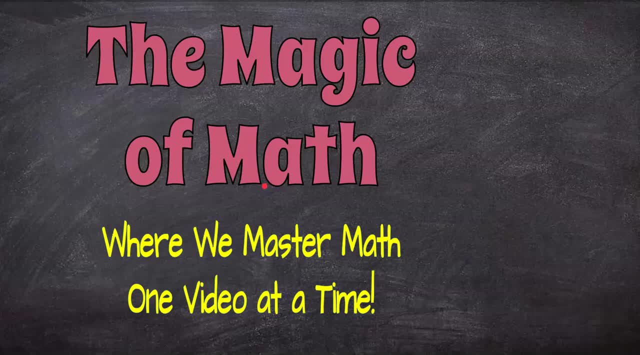 absolute value equations. I hope you'll come back for a future video where we're going to solve more complex absolute value equations. And that is it, The magic of math, where you are mastering math one video at a time. I hope you'll subscribe.